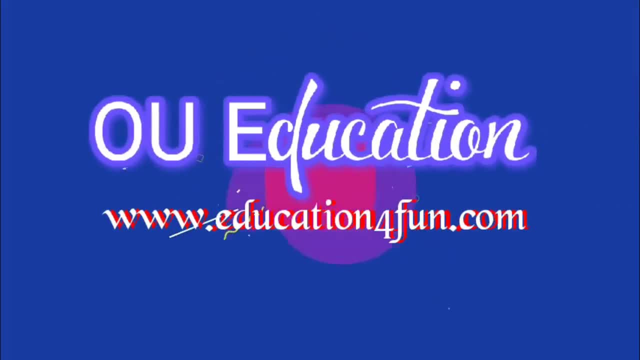 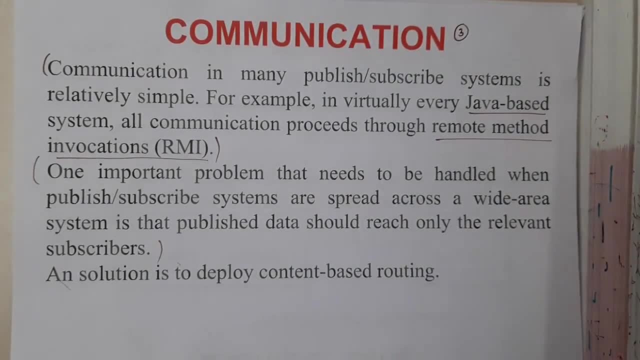 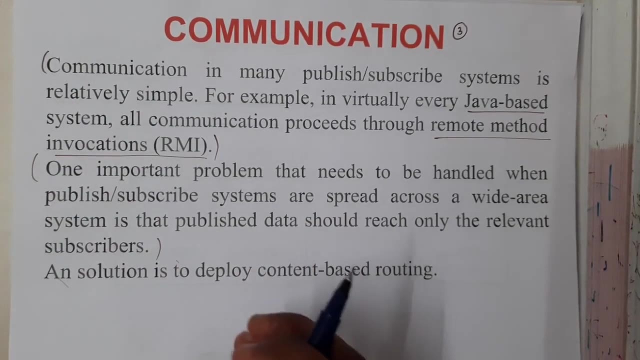 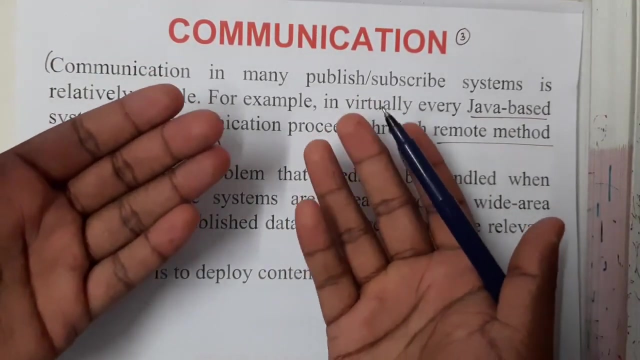 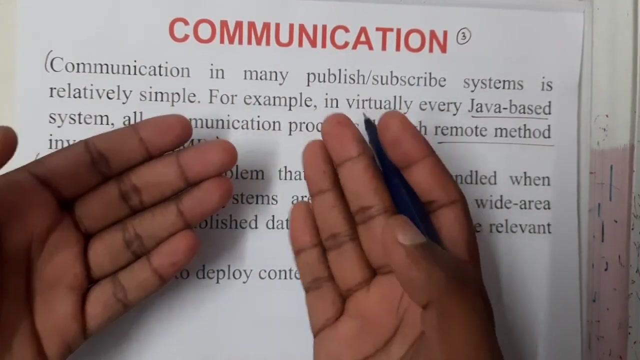 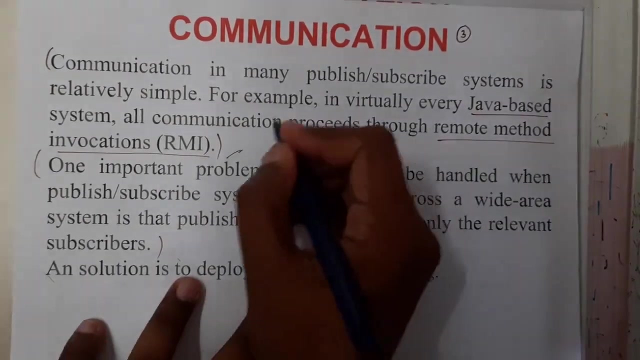 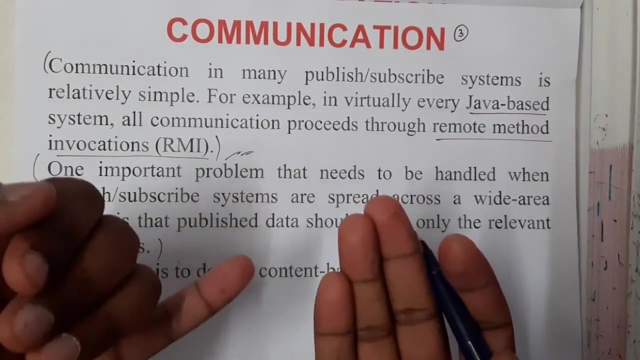 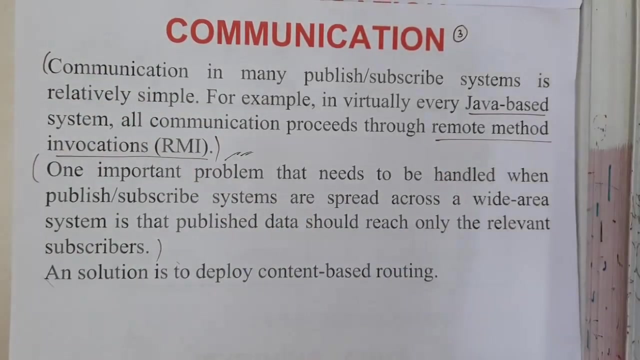 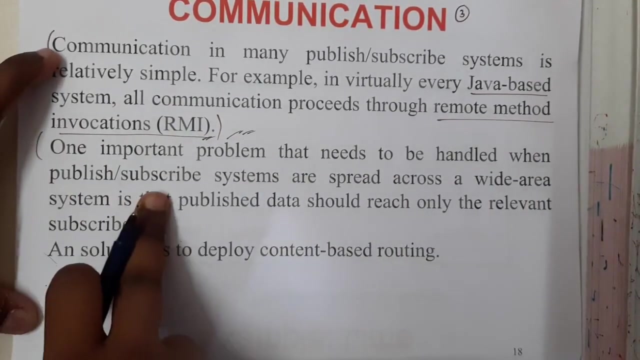 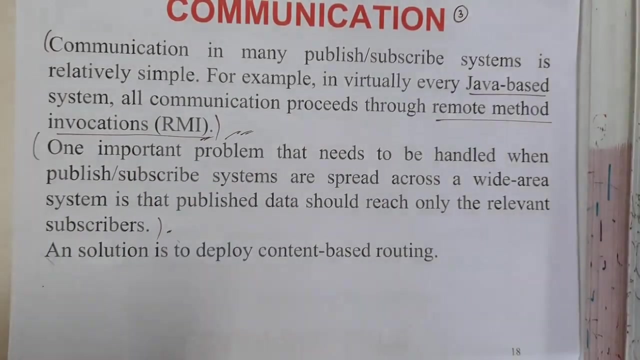 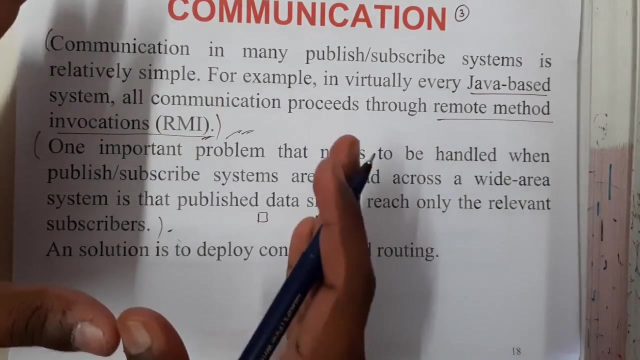 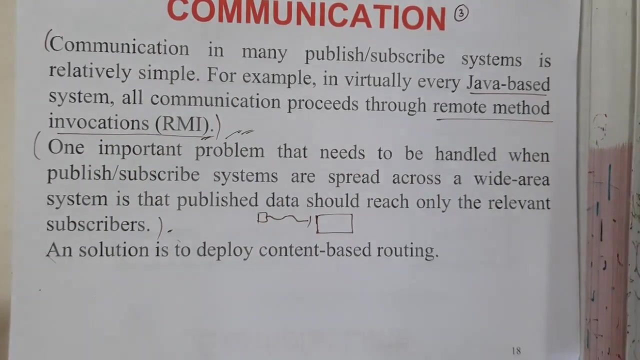 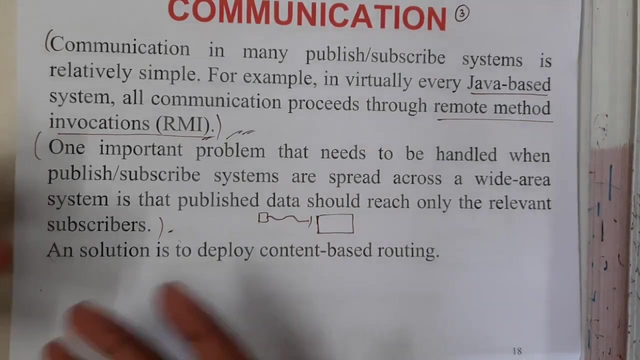 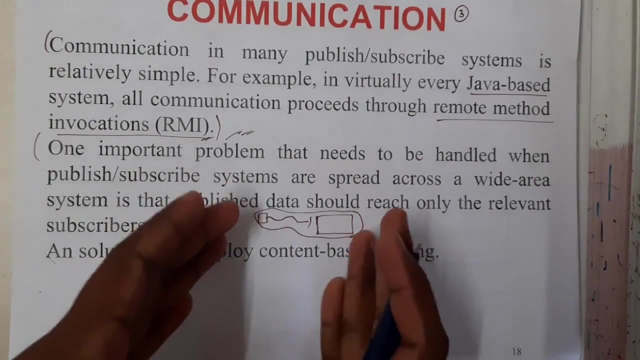 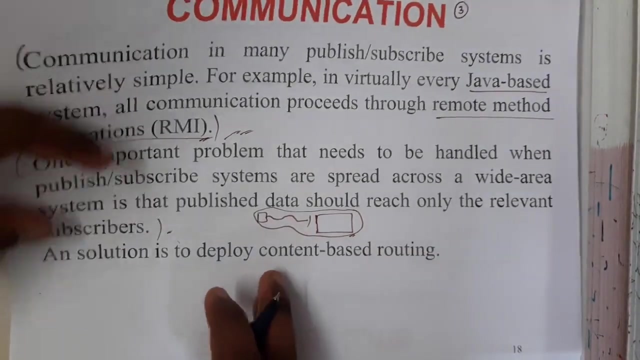 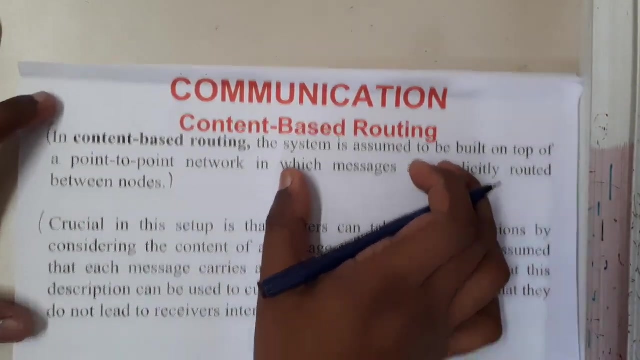 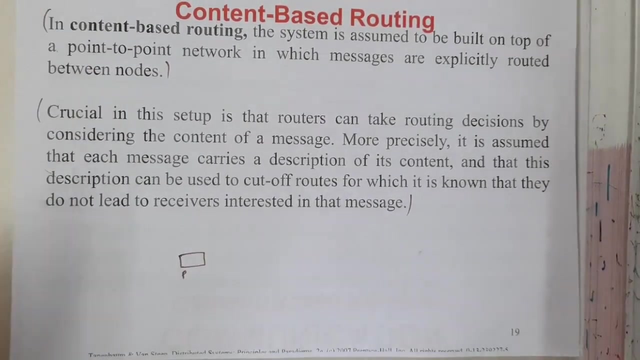 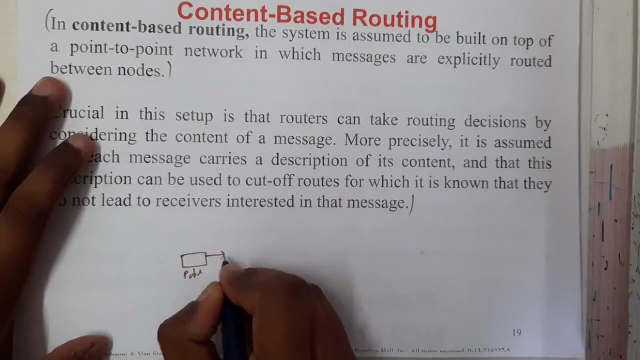 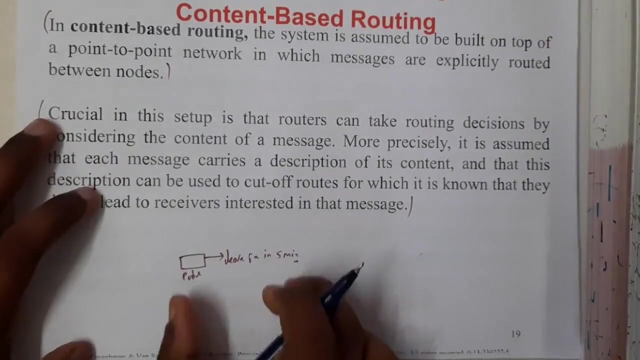 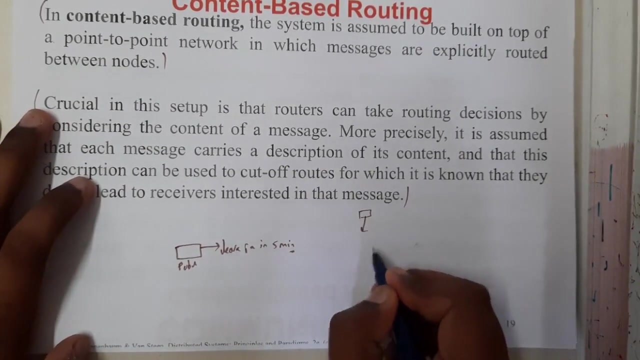 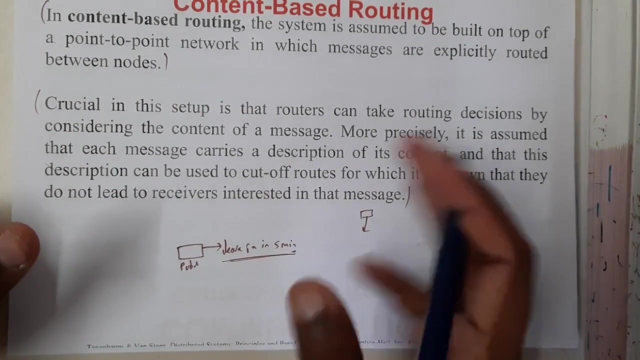 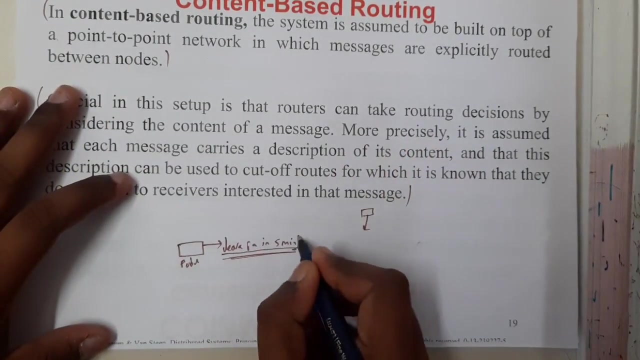 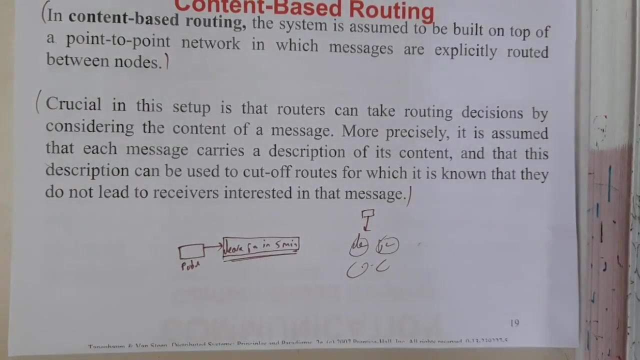 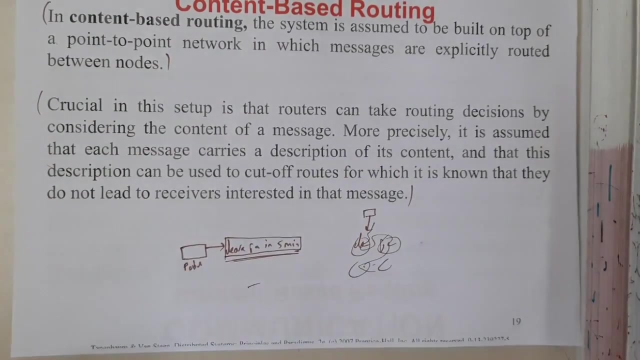 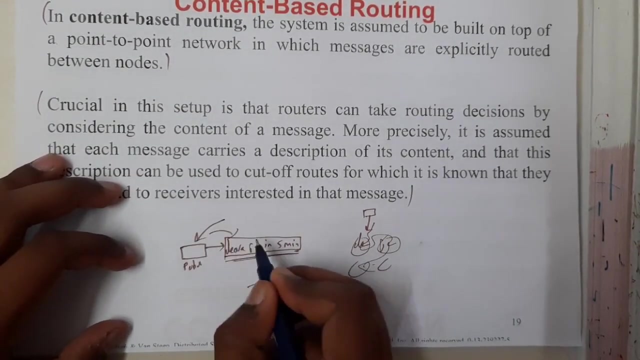 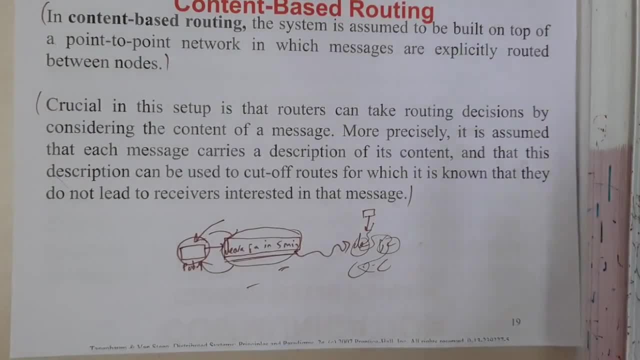 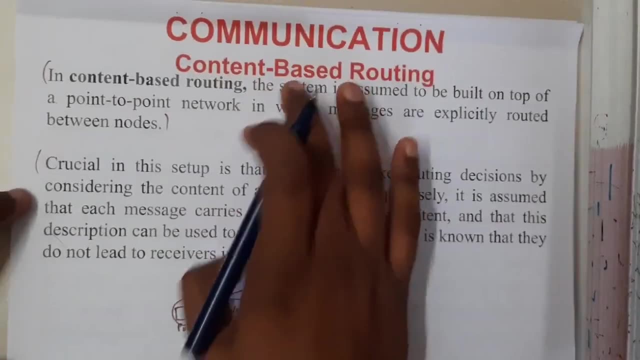 that situation, it is a traveling to the nearby subscriber who wants it. so this is nothing but content-based routing, guys. guys, i think a few of you might be confused, but once we are going through the definitions, you'll be having a clear idea, guys. so that's the reason why i gave you the 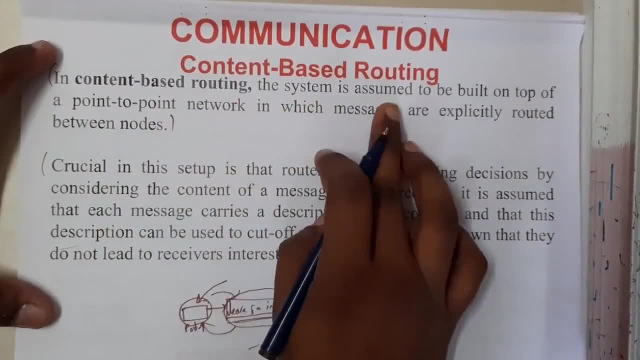 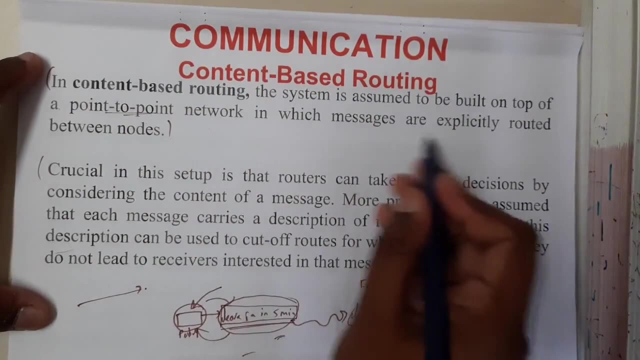 example: first, okay, yes, so in content-based routing the system is assured to be built on top of a point-to-point communication, so one person to another person, some kind of notification. you can say, okay, in that way it will be sent. okay, through the nodes. crucial in this setup is that. 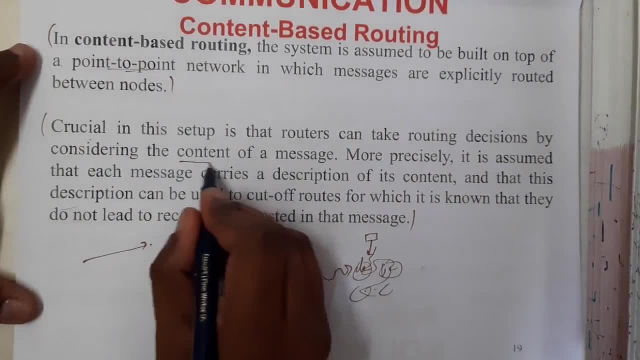 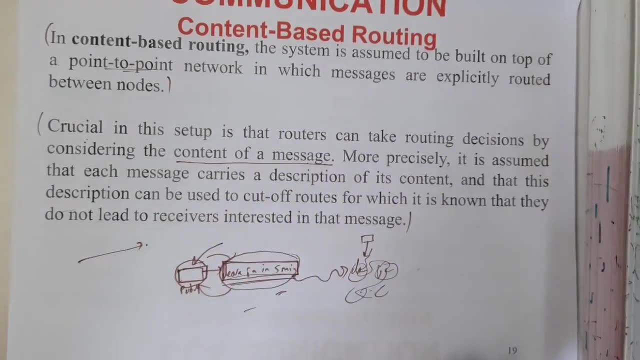 router can take routing decisions by considering the content of the message. so here, instead of message, i am taking the example of video, and about the video or about the message is written as a title. okay, so, most preciously, it is assumed that each message carries a description, so this: 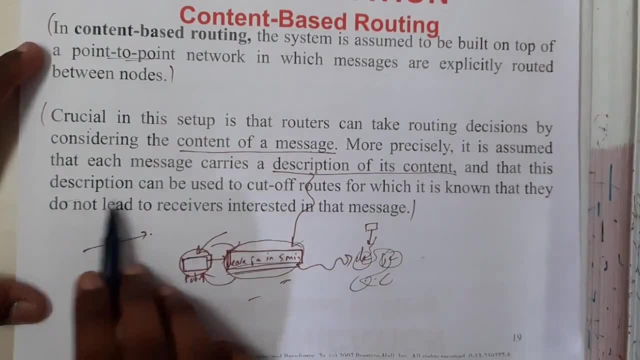 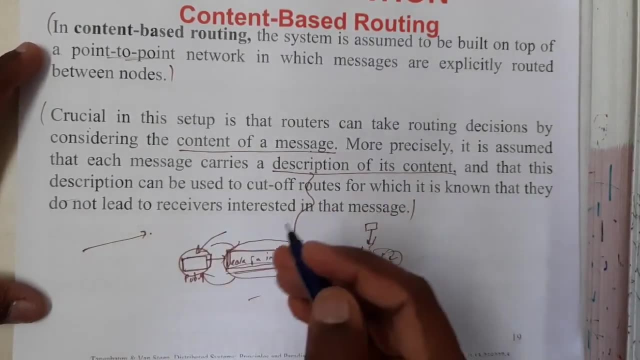 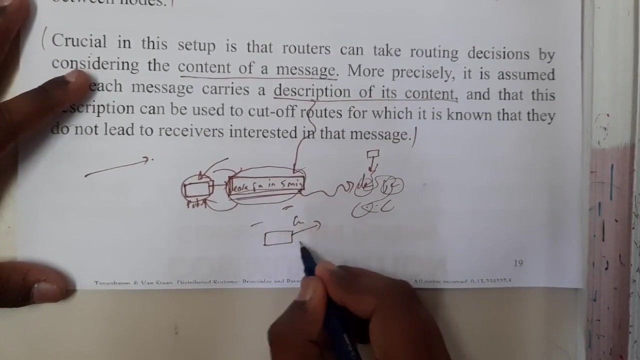 description is nothing but our title, guys. okay, and this description can be used to cut off routers for which it is known that they do not need, or they do not need this type of content. so assume that the node has started here, guys. so there is a one game, one side that is nothing but gaming. another side is: 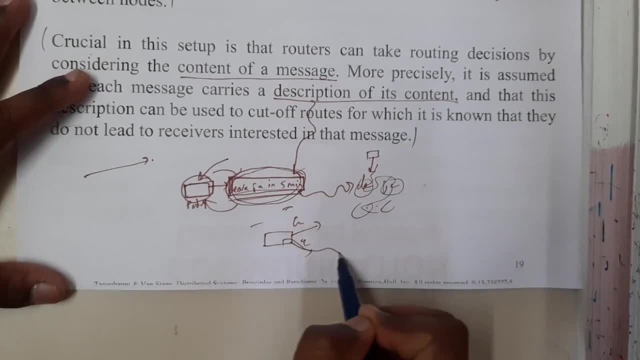 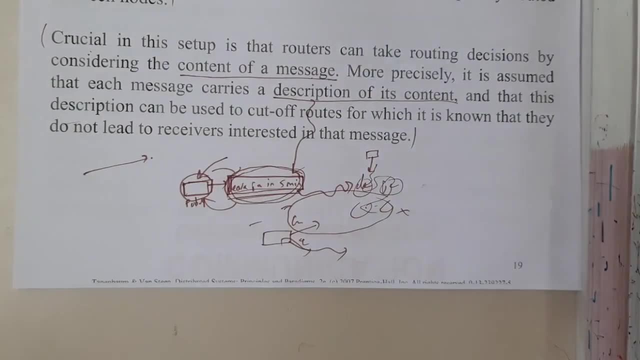 education. so if this is the video, in which path it will go, guys? it will go in this path, right education path, and this whole path will be omitted. so this is nothing but content-based routing. so, based on your content, you are right, routing your packet or your video or your message. so that is. 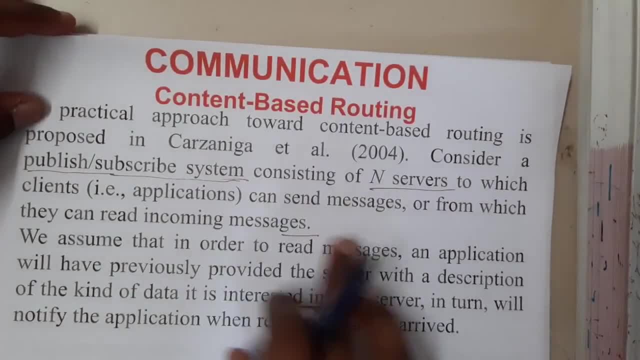 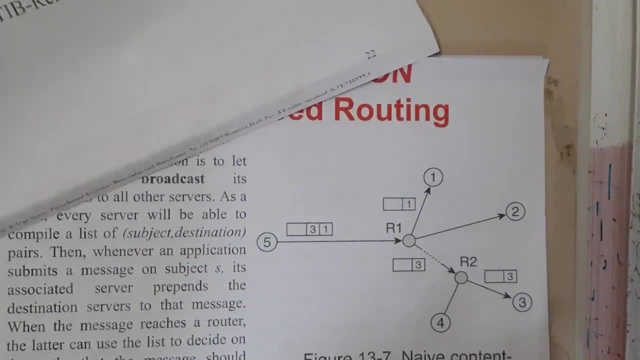 content-based routing, guys. okay, okay. so this is an example, guys, you can just go through the example. okay, okay, this is also one more example here. we are having n servers and we are transmitting it, okay, so now i hope everyone got some basic idea about how the content-based routing is done, right. 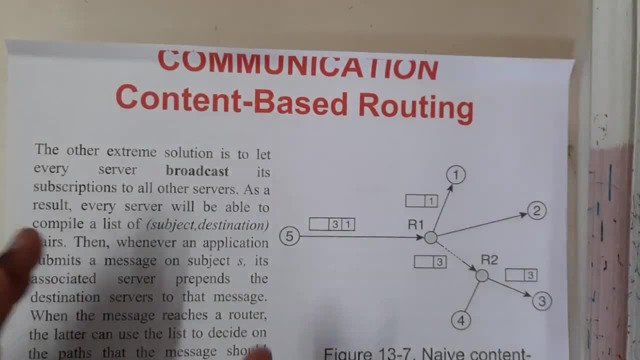 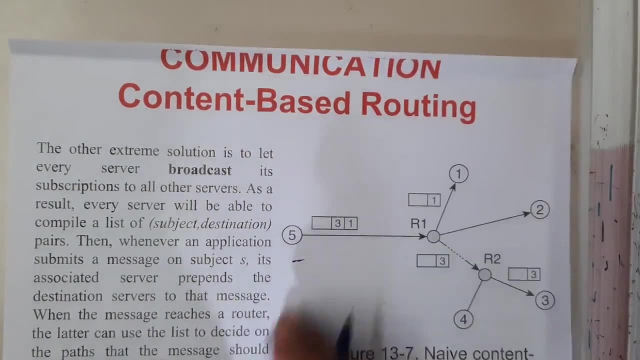 yes, so you might be having it okay. so then only for them. if it goes, then there is no upgrade of subscribers or everything right. so only they will be watching, right? yes, so that is the reason why we will also have the broadcasting mechanism also. so basically, in this situation, once you enter into 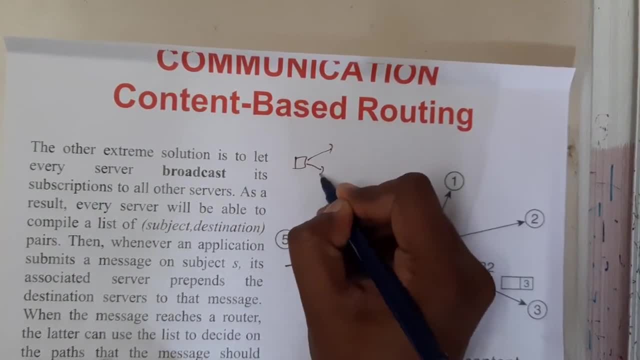 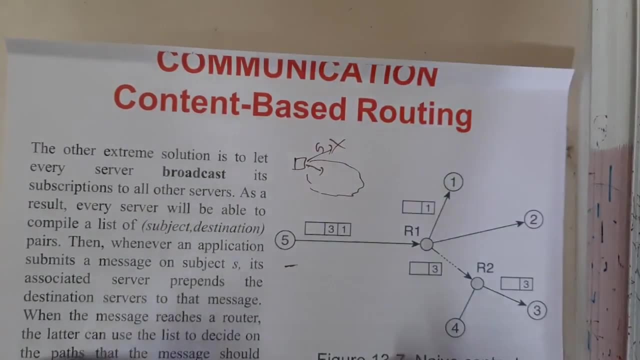 the education part. so, basically, here we started, here there is gaming and here there is education, right, yes, so once you avoid it and you start playing games, and you start playing games and you start playing games, the gaming. and if there are very less number of educational channels or educational students, So in that situation, 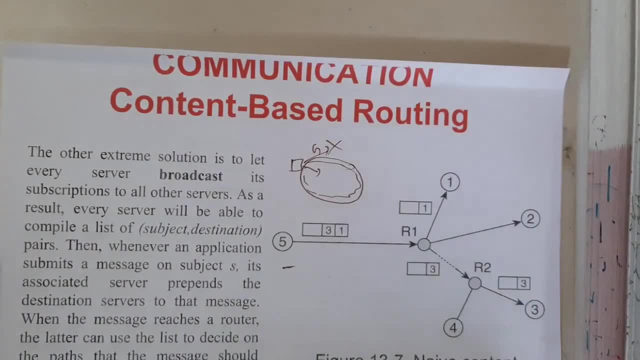 you can broadcast your message here. So basically it will go to everyone. It might be a spam, but it can. there is a chance also, Okay, So in this way. So here 5 has sent to router 1 and here from here, everyone.